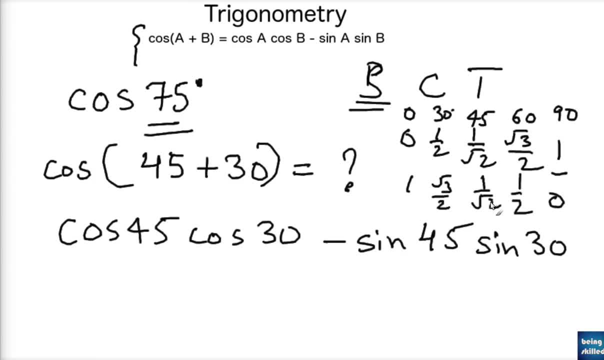 1 by 2, 0.. So what are the desired values? Cos 45 is. so these are the values of sine, these are the values of cos. So cos 45 is 1 by root 2, then we have cos 30, which is root 3 by 2 minus sine 45, which. 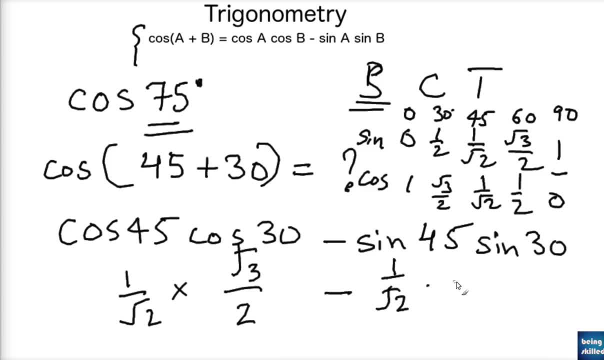 is 1 by under root 2, sine 30, which is 1 by 2.. So we have under root 2, under root 2. and minus 1 by 2 and root 2.. So we have and root 3 minus 1 upon 2 and root 2, which is the desired value. 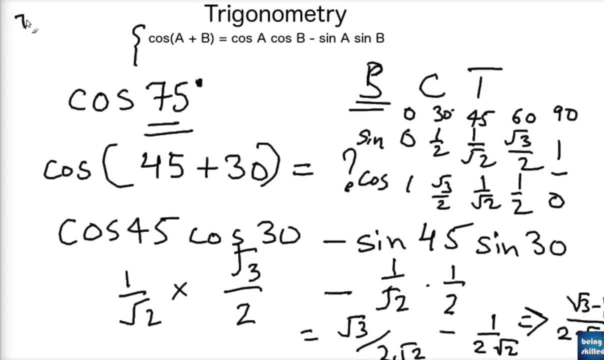 So, in case you want to solve it further, and root 3 minus 1 to root 2 into root 2, into root 2, which happens to be, and root 6 minus and root 2 upon 4.. So it is suggested that you shouldn't have and root values in denominator. 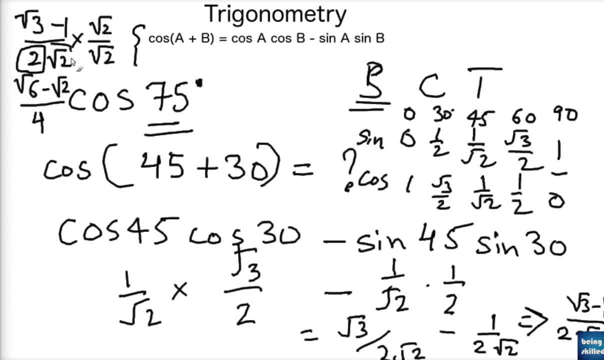 So you can just multiply and root value which is and root under root It is suggested that you should have. you shouldn't have under root 2 values in denominator. So you can just multiply the numerator and denominator by the values which are under root. 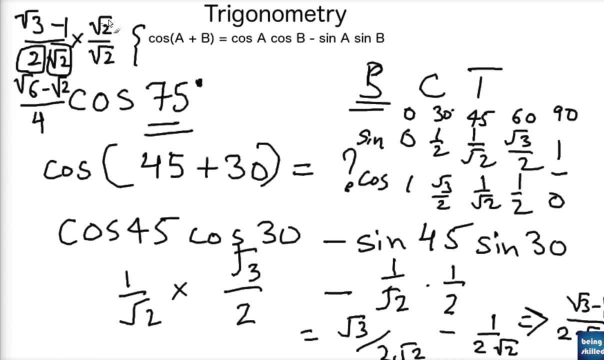 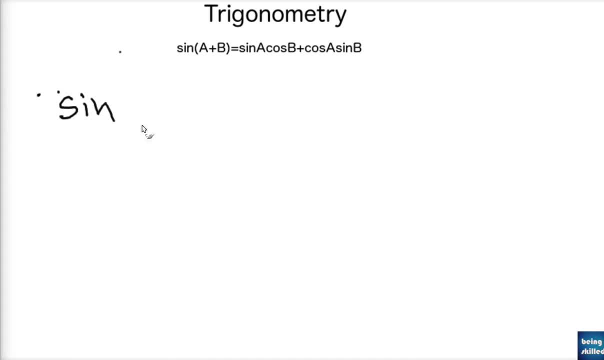 So in case, in this case we are multiplying it by and root 2.. So the final value is and root 6 minus and root 2 upon 4.. Now suppose we have sine 75 and we want to calculate its value. So we know that. 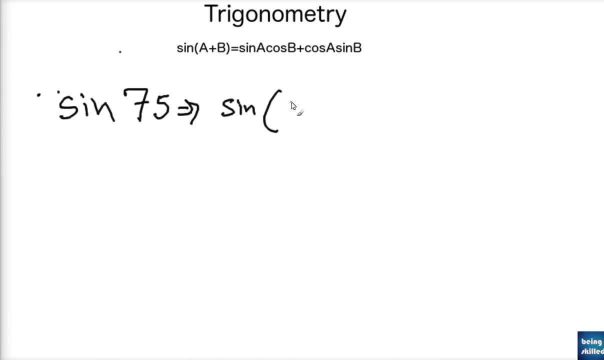 Sine 75 can be written as 45 plus 30. So we just have to calculate its value. So we have to. we remember that sine a plus b equals to sine a cos b plus cos a sine b. So we can just under the values. so sine 45 cos 30.. 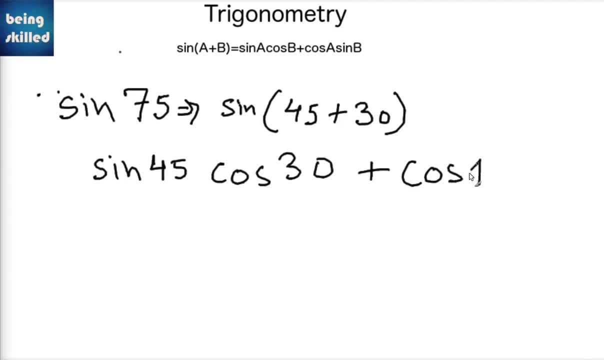 So we can just under the values, so sine 5 plus cos 45, sine 30.. So we remember that 0, 1 by 2 and by root 2, root 3 by 2, 1, 1 and root 3 by 2, 1 by 2, 1 by 2, 0.. 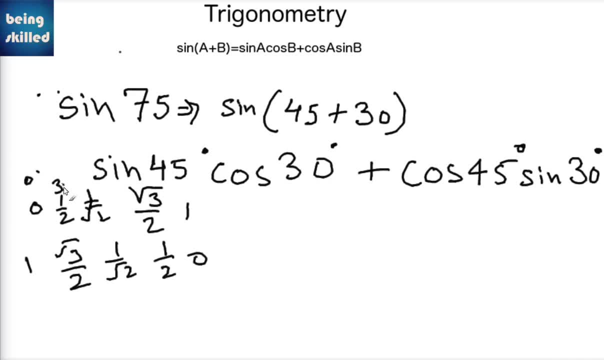 This is 0 degrees, This is 30 degrees, This is 45 degrees, This is 60 degrees, This is 55 degrees degrees and this is 90 degrees and this is sine. and this is cos so we um, so the values which we. 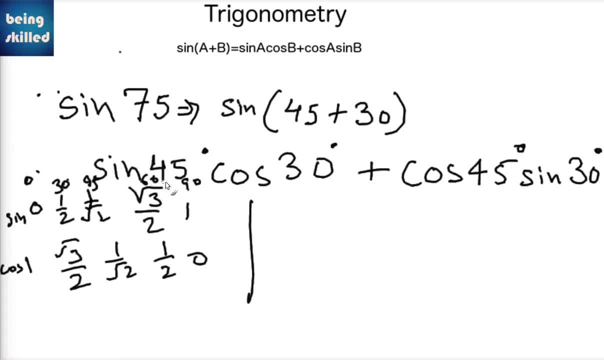 have um for sine 45 is 1 by n root 2, cos 30 is n root 3 by 2, plus cos 45 is 1 by n root 2 into uh we have sine 30, which is 1 by 2, so n root 3 by 2 root 2 plus 1 by 2 root 2, which is 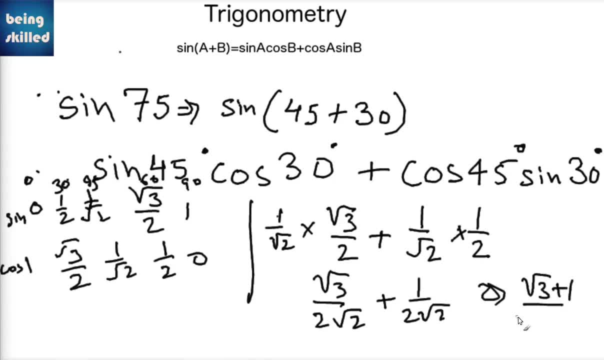 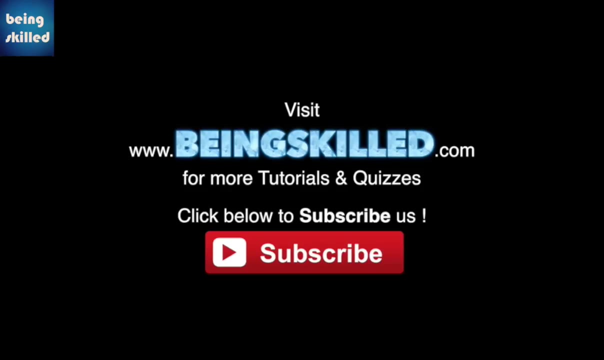 n root 3 plus 1 by 2 root 2, multiplied by 2 root n root 2, so we have n root 6 plus n root 2 upon 4. so this is the desired value of sine 75.. thank you for watching the tutorial. please don't. 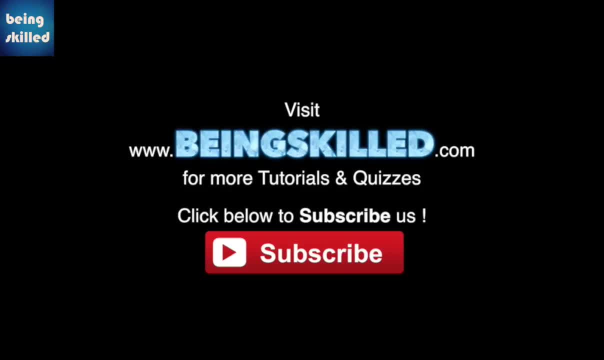 forget to click on the subscribe button for receiving more updates from being skilled.